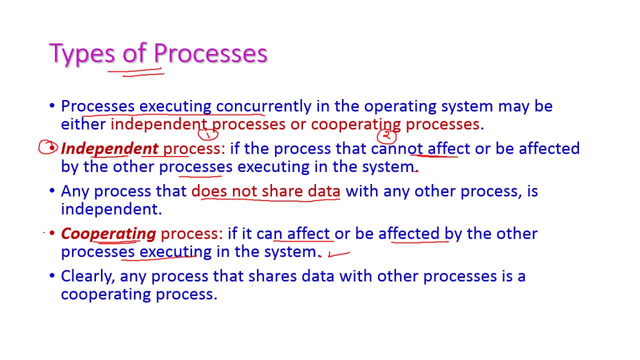 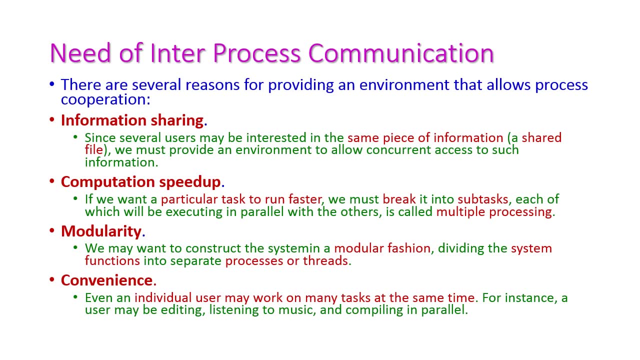 okay, so the processes can share the data with other processes, which are called as cooperating process. and next let us see what is the need of inter-process communication. here there are several reasons between the process to communicate each other. the first one is information sharing, second one is computation speed up, and third one is modularity. and fourth, 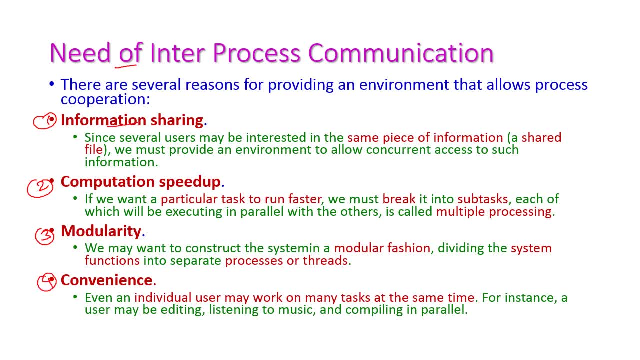 one is convenience. okay, first let us see what is information sharing. information sharing means some piece of code may be shared by more than process processes. hence we need to create an environment to share such files or information that should be common for all the processes, okay, so that all the process can concurrently access those. 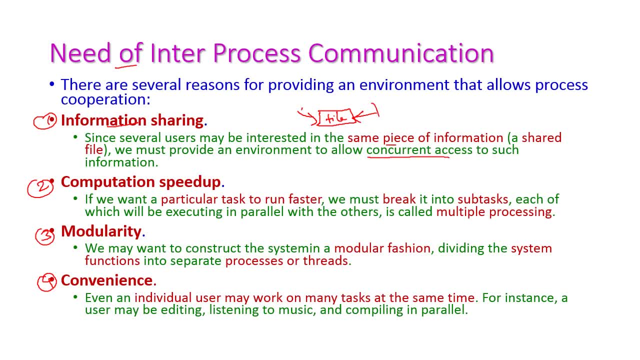 piece of information, then this is called as information sharing. and second one is computation speed up. so computation speed up means if there is a big task that should be executed faster, then that task should be divided into subtask- so many subtask, suppose. if it is our task, this is: 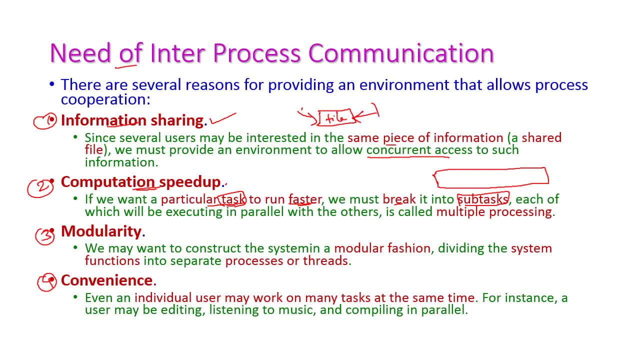 very big and this should be run very faster. hence we have to divide that into subtask. this is subtask, and all those subtask should execute parallel, and this is called as multi-processing system. okay, and by this way we can increase the speed of our computation. and next one is modularity. 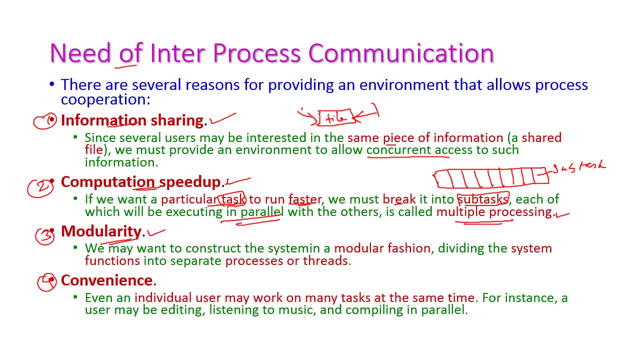 okay, here we have to construct our system into modular fashion, that is, the system's functions will be separated and that will execute a separate process or threads. this is called modularity. modularity means this is our system and the system functions will be separated and and each function is called as a module. the modules will be, each functions will. 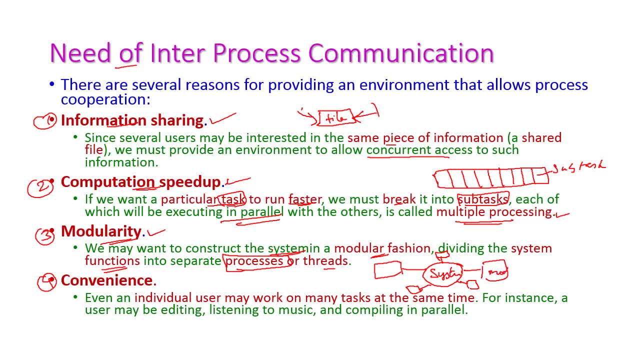 be separated and that is called as module module, module 1, module 2 and the fourth one is convenience. convenience means a individual user can execute more number of tasks at a time. for example, the user may use a document file, they may use the media player for listening music and compiling the Java program or 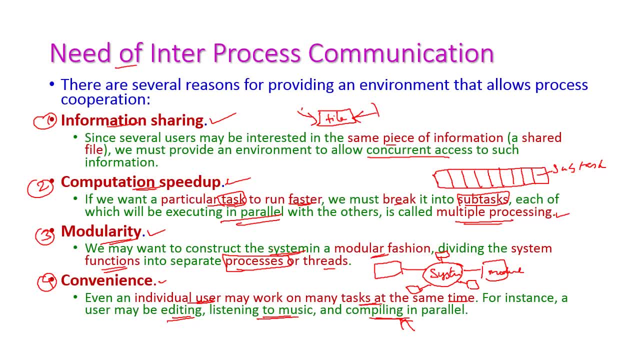 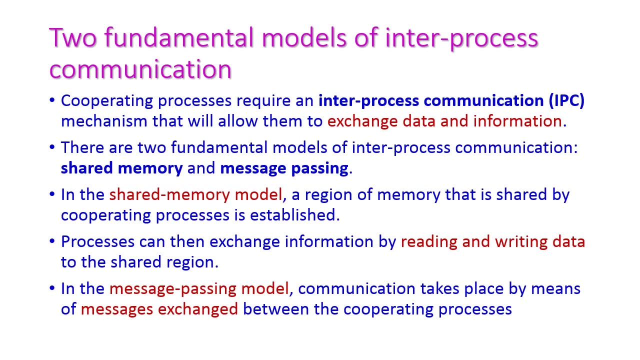 any other program in parallel. okay, so the user can execute more number of programs at a time. so we need to create a convenient environment for the users also. okay, these are the need for the inter process, community communication, and next let us see the fundamental models of inter process. 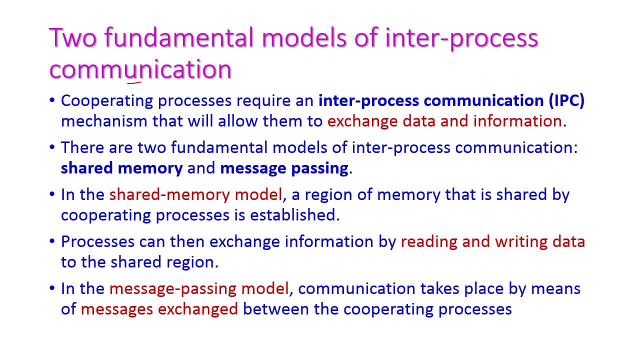 communication. here the process, more number of process- can communicate with each other and they need to exchange data and information between each other. here the two models are: the first one is shared memory and second one is message passing. shared memory means a region of memory that is, a portion of memory is. 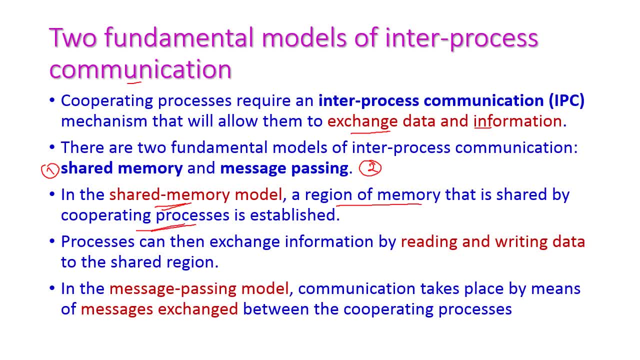 shared by the process, and the process can exchange information by reading and writing the data on the shared region. okay, see, this is the memory and this is process one and this is process two. this portion will be common and in this portion, both process one and process two can read and write the information, and next one is message. 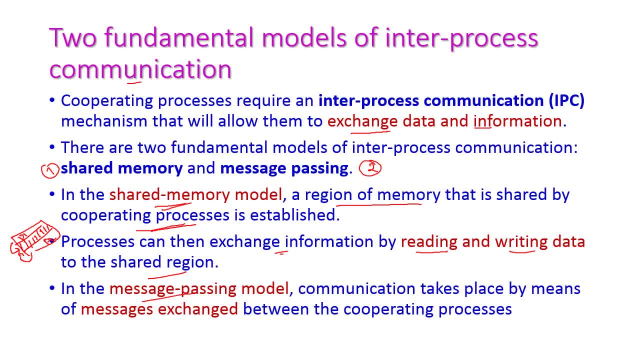 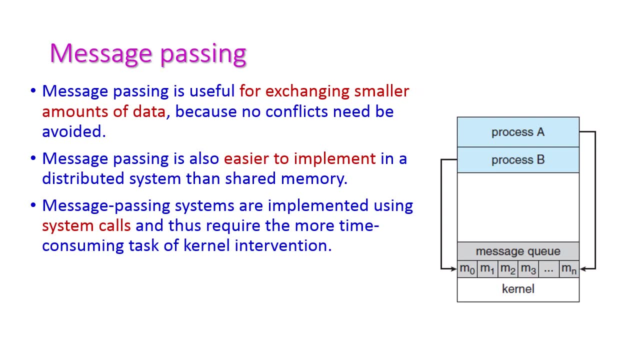 passing model. see: in the message passing model the communication will be take, expressed by means of exchanging the messages between the processes. Let us see all those things in detail. First one is message passing. Here, message passing is useful for exchanging smaller amount of data between the processes. Hence the conflicts will be avoided, and it is 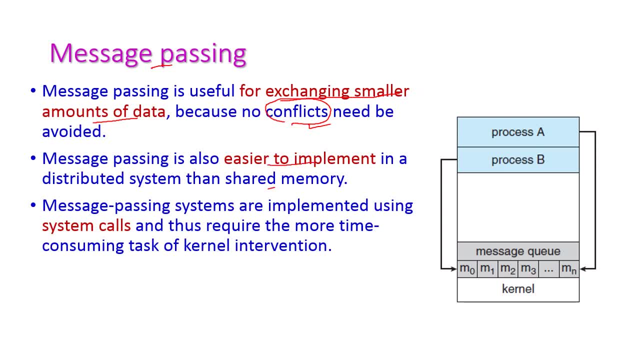 also easy to implement when compared to shared memory, and the message passing will be implemented by using the system calls Hence it required some more time when compared to shared memory access. Okay, and this is the simple diagram for message passing. Here we are having process A and process B. If process A wanted to send some messages to process, 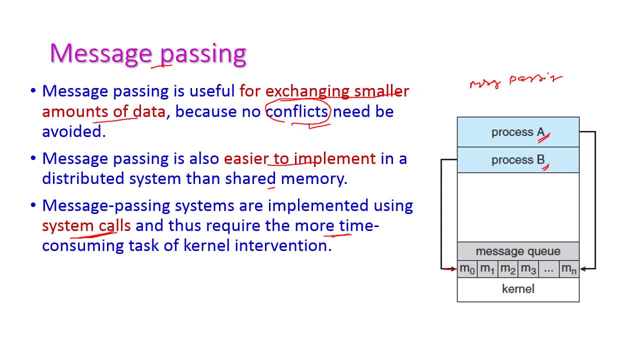 B means it will send the message to kernel. Then the kernel will send this particular message to process B. That is the process A send a message to message to kernel and the kernel transfer this message to process B. So this is how the message passing will be taken place. Next let us see the 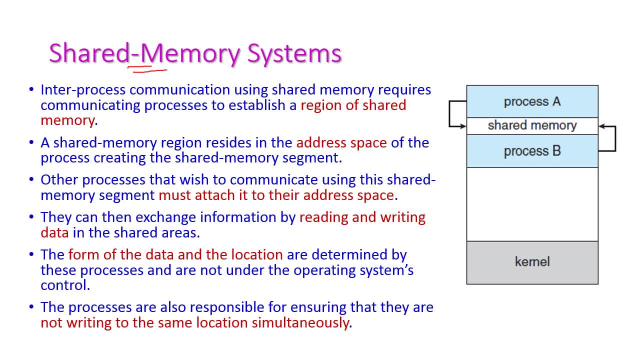 shared memory system. Here a portion of the message passing will be taken place by the kernel. So this is the shared memory. A region of memory will be shared by both the process. Then this is called as shared memory system. Here the shared memory will be received in the address space of the processes. 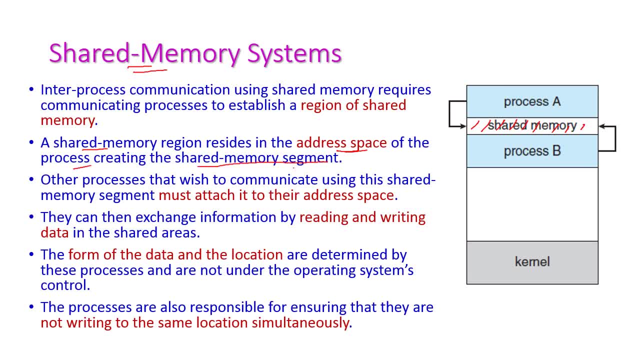 they are creating in the shared memory segment. So in this portion itself the memory will be reserved for both the processes. And if the other process wanted to communicate by using shared memory system, then this is called as shared memory system. So in this portion itself the memory will be. 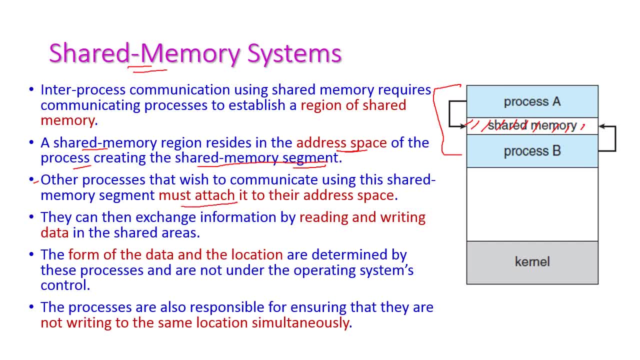 reserved for both the processes And if the other process wanted to communicate by using shared memory segment means they need to attach the address spaces. This address space should be attached to other process also. Then only they also access this shared memory And the address space will be. 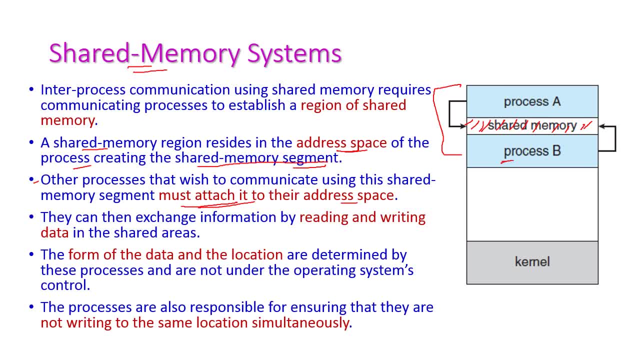 exchanged by the both processes by reading and writing operations. So, for example, the process A can write something, This will write something and the written data will be read by process B. Process B will read the data, And the form of data and location are determined by this process only not under the control of operating. 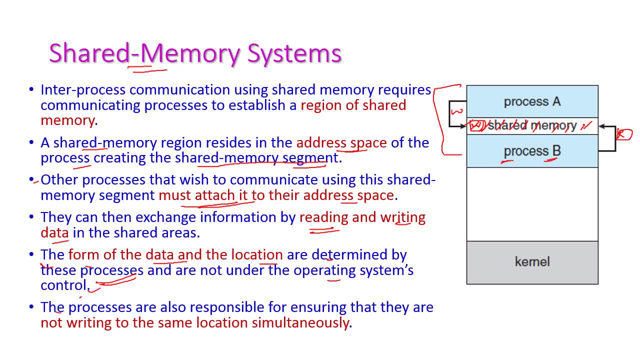 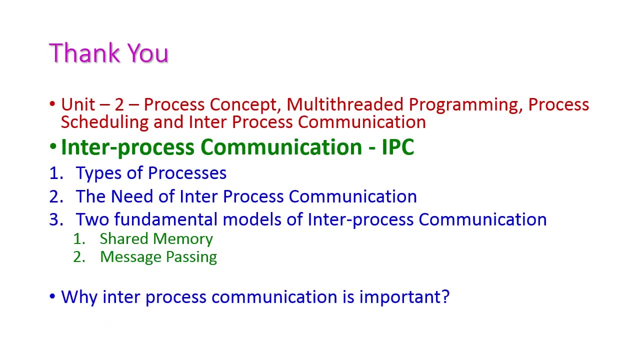 system And this process also responsible for ensuring they are not writing to the same location simultaneously. This is important, Otherwise conflict may occur. After this we have seen the inter process communication that is, IPC Under this types of processes and need for inter process communication. after that we have seen the two fundamental inter processes communication models.